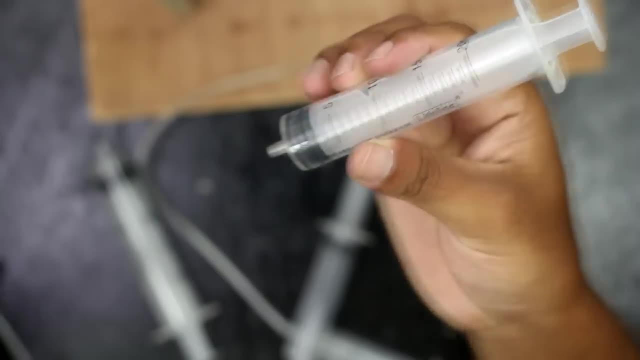 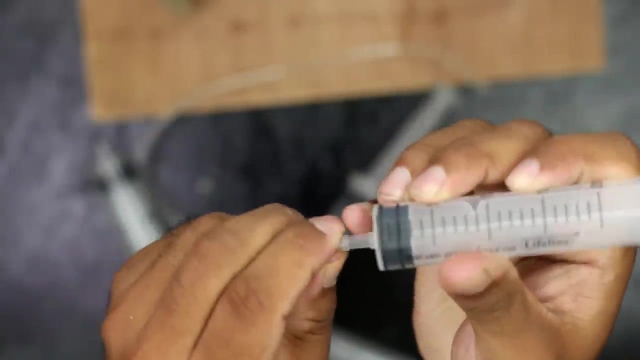 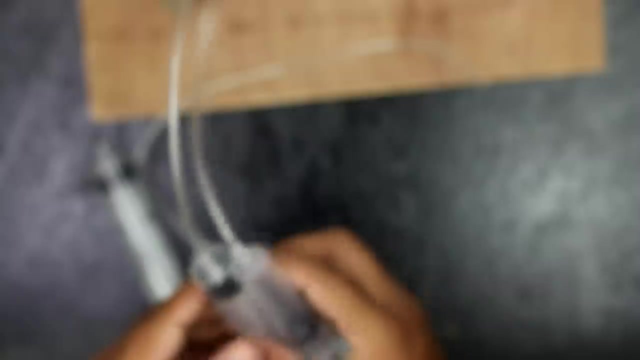 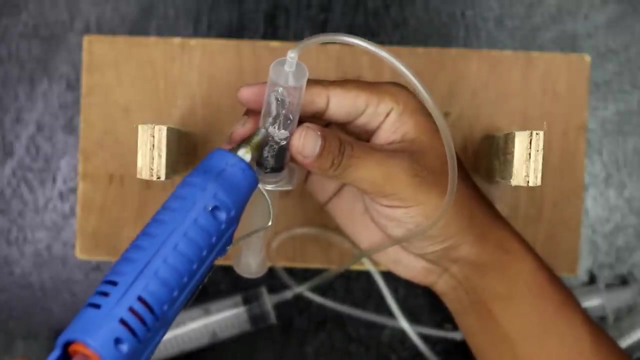 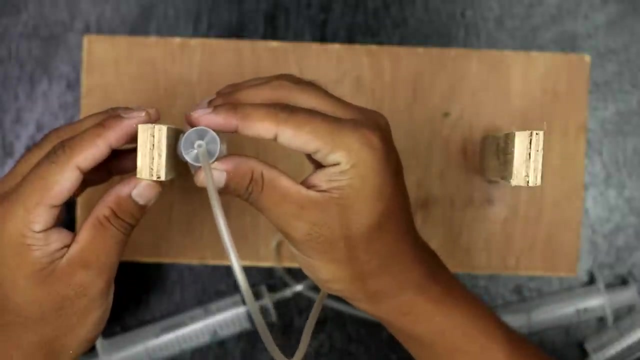 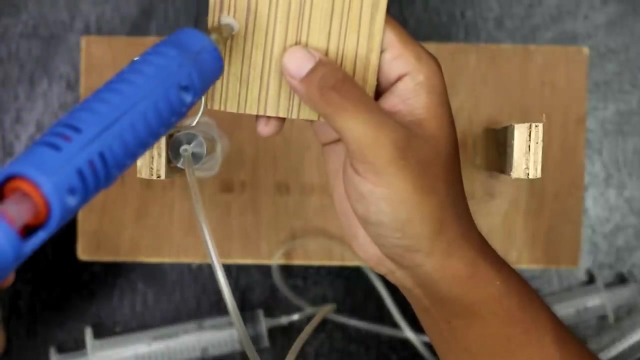 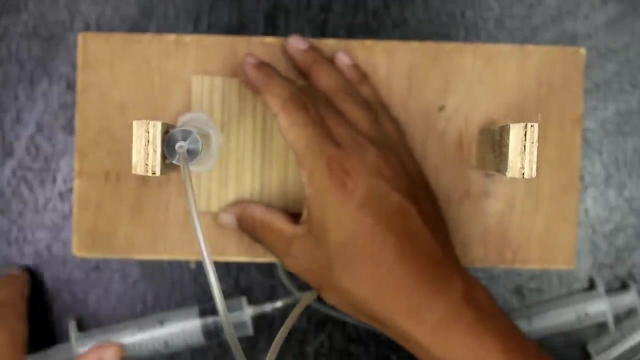 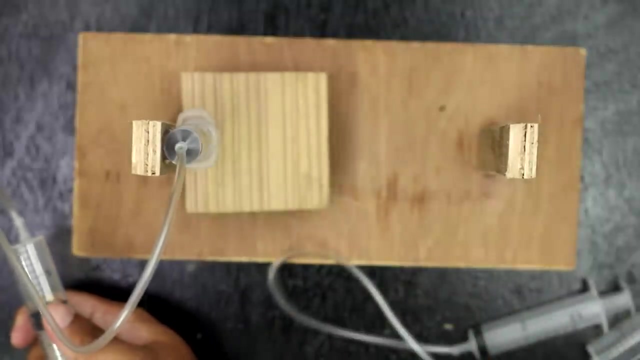 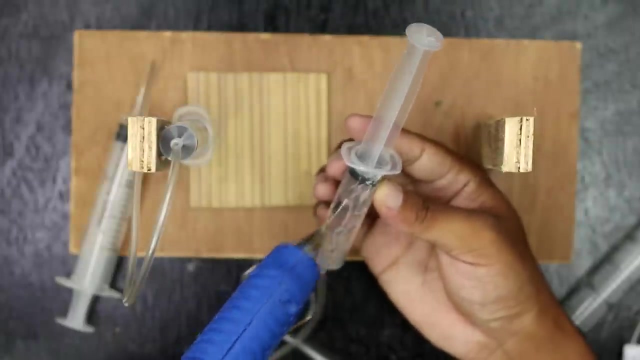 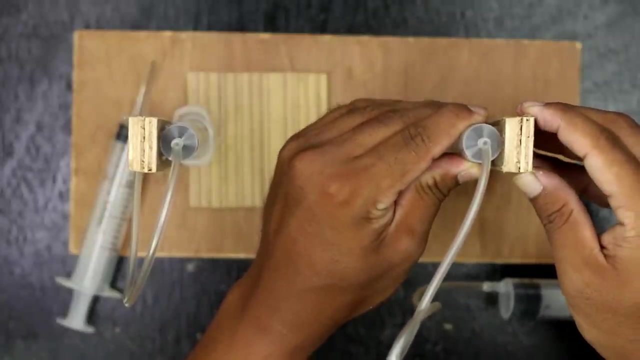 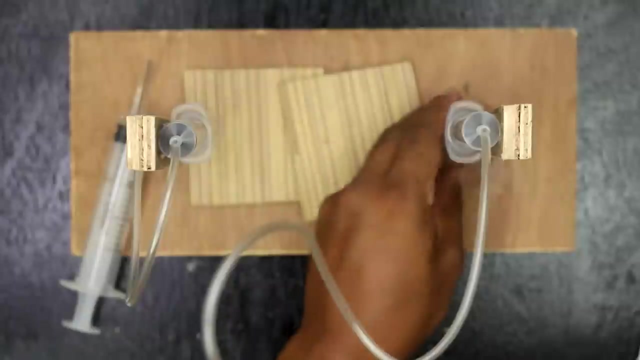 on one syringes, Glue, 10ml syringes at the side of stand and thin plywood at the base so that when we press syringes this base moves up and down as a lift. 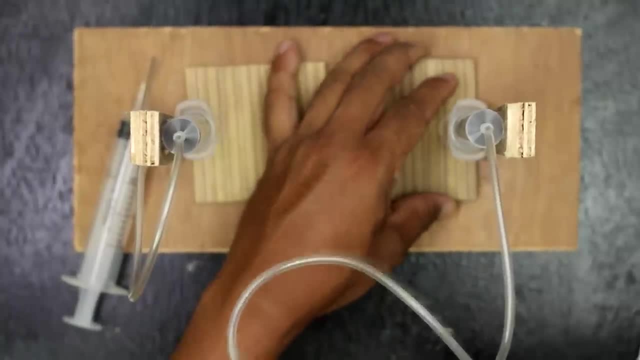 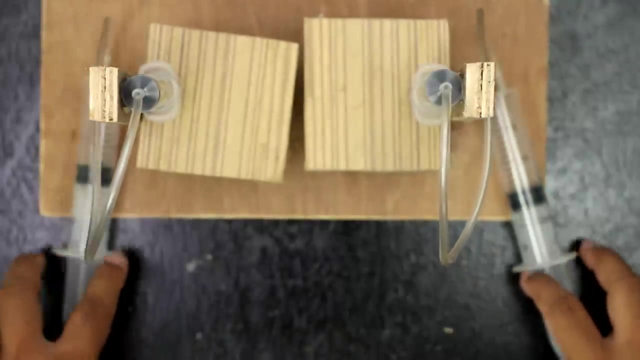 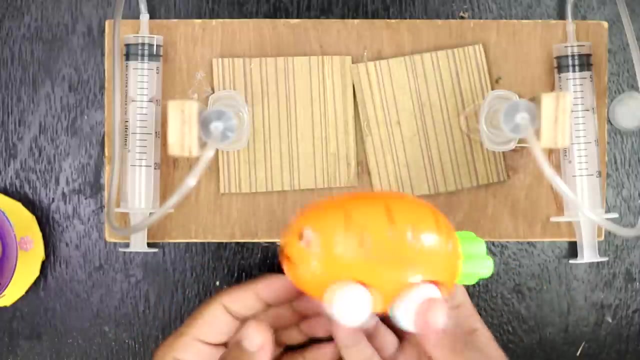 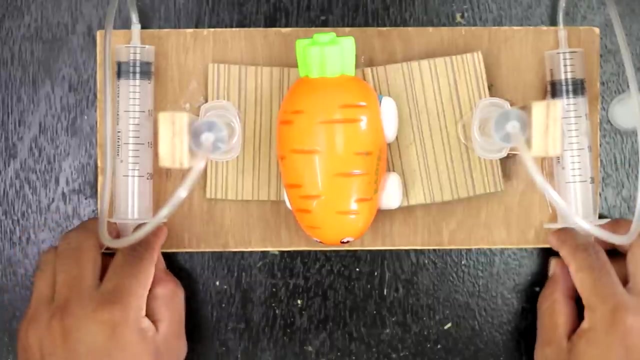 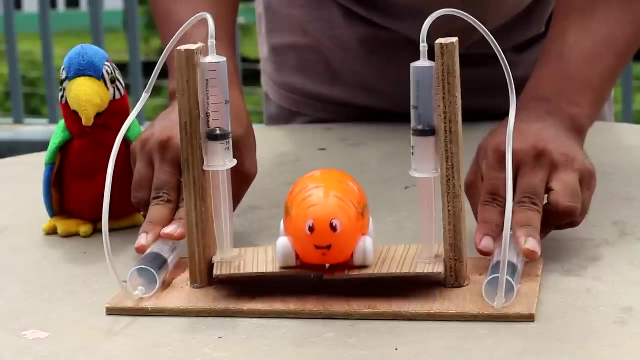 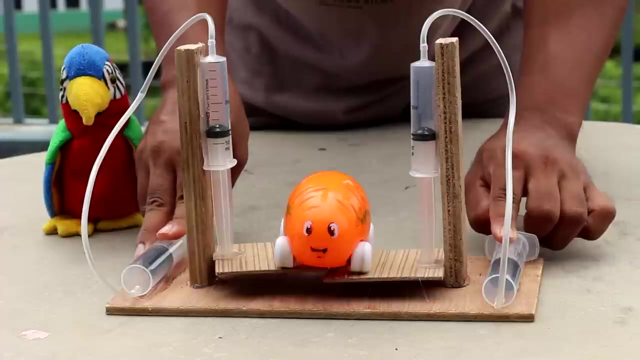 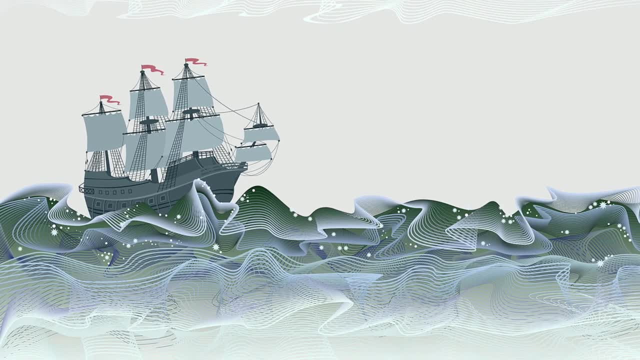 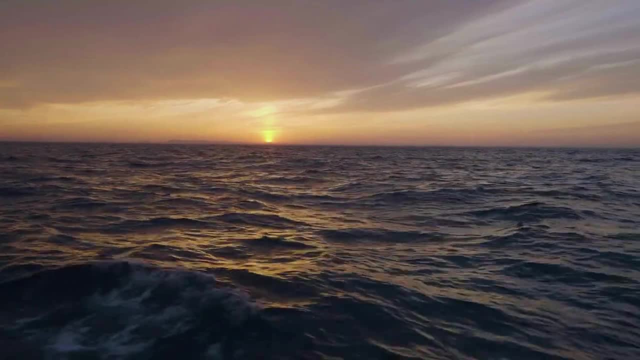 In ancient times, sailors realized that certain winds are always present at certain locations on earth. In fact, many sailors became rich by using the trade winds to travel from one city to another. Why do we have these winds on earth? Welcome to MooMooMath and Science and Global. 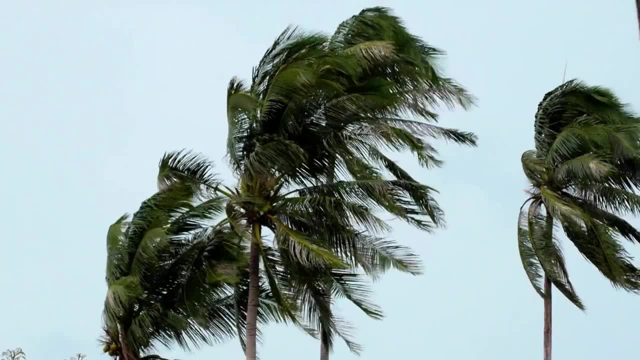 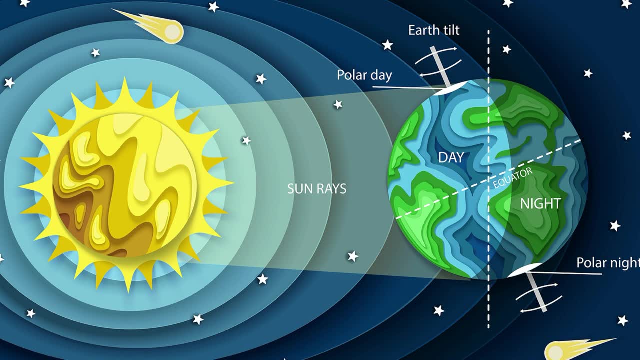 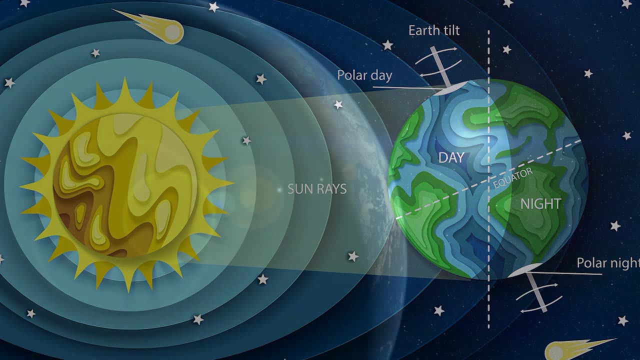 Winds. In order to understand global winds, we need to learn some basic facts. Due to how the earth tilts on its axis, the sun's rays strike the earth at different angles. This results in unequal heating of the earth's surface. For example, the equator receives more direct sunlight.